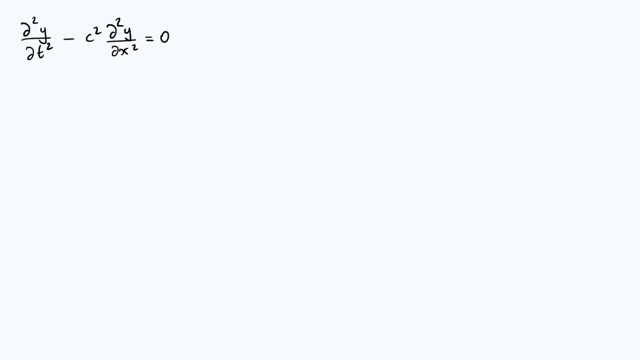 solution in advance, whereas taking the Fourier transform is a pretty standard method when you're solving a partial differential equation. so that's why I'm choosing to do it this way Now, because this equation contains derivatives both with respect to time and with respect to. 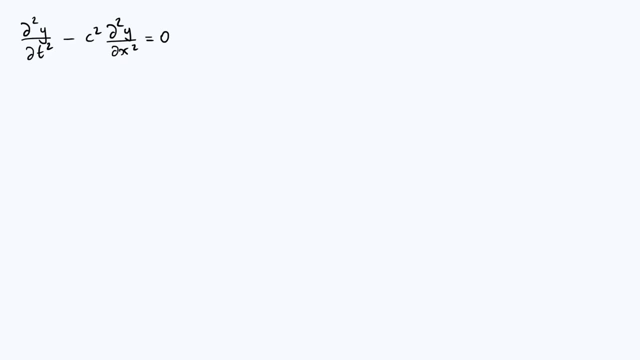 position x, we've got to choose whether to take a spatial Fourier transform or a temporal Fourier transform. Now, either of those will work, but I'm going to choose to take the temporal Fourier transform, and so let me just show you the definition that I'm going to use. 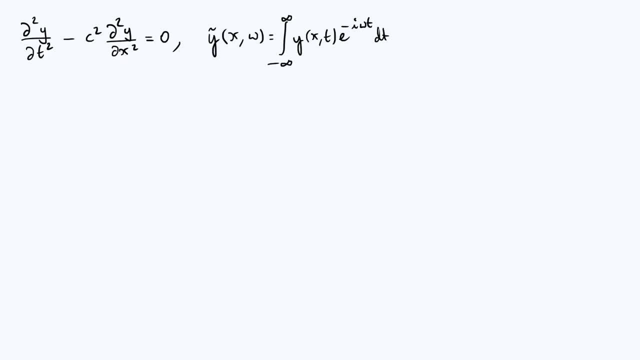 Because there are various definitions around. So my y tilde, which is the temporal Fourier transform of y, is just the integral of y times e to the minus i, omega, t with respect to time, over all values of time. Under this convention, the inverse Fourier transform, 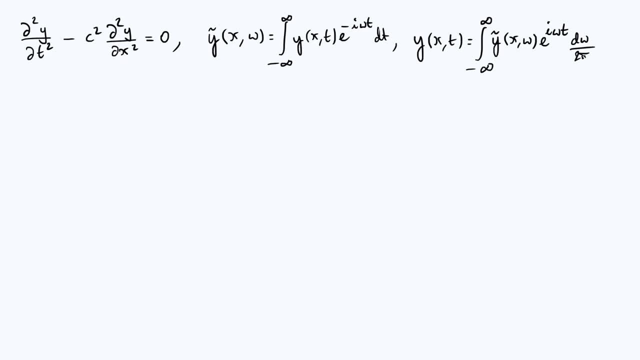 in other words, to get back to y as a function of x and t is an integral over all values of omega of y. tilde times e to the i omega t, but then you've got to divide by 2 pi as well. So let's see what happens if we actually go ahead and take the Fourier transform. 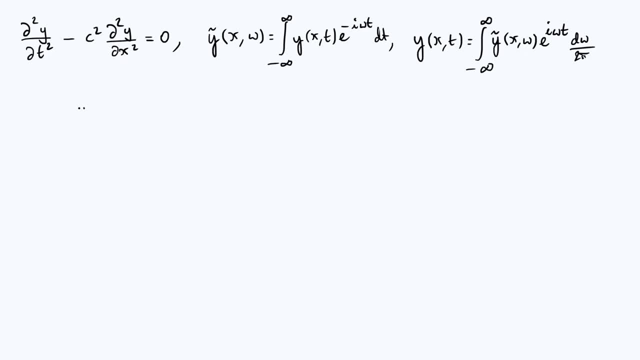 of our original PDE. Now, what I mean by that is you just take the whole equation which I'm going to write as dot dot dot, you multiply the entire equation by e to the minus i, omega, t, and then you just integrate both sides of your equation over all values of time. 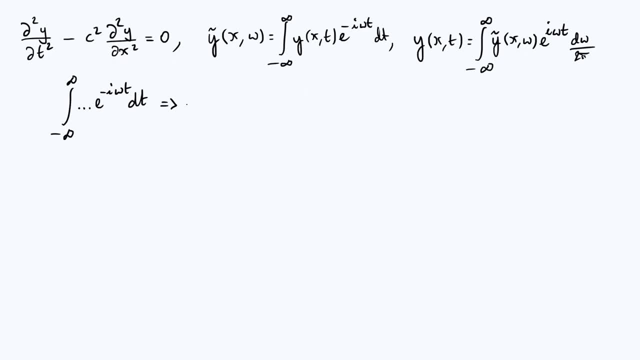 Now the reason this is a useful thing to do is that differentiation in real space corresponds to multiplication by i- omega in Fourier space. Now, that's a result that I derived in my last video, so you can have a look at that if you're interested. 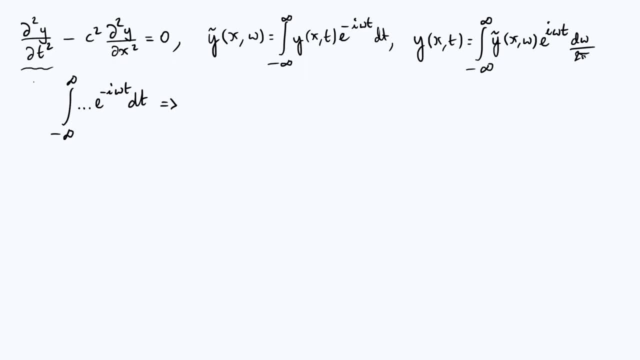 but basically what that means in practice is that this first term in our partial differential equation, d2y by dt, squared in Fourier space, is just going to be i, omega squared times y, tilde of x and omega, right. So this is why Fourier transforming differential equations is useful. 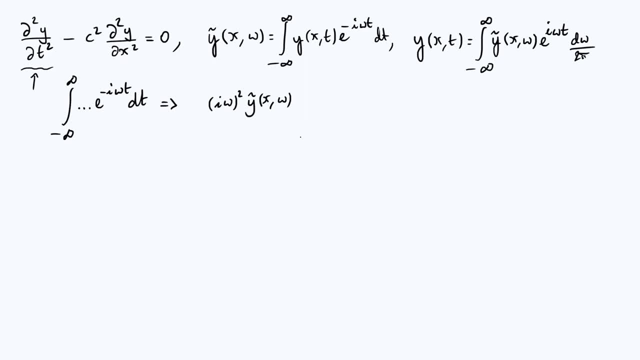 because it turns derivatives into just multiplication. The second term in our original PDE we can't use that trick with because we took the, the temporal Fourier transform, and that's a spatial derivative. So we're going to have to leave that second term as minus c squared and then just the second spatial derivative, d2. 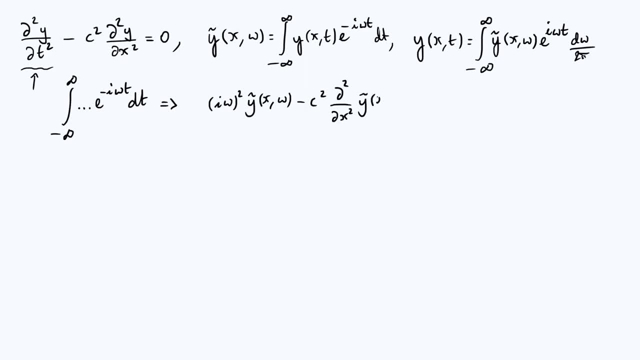 by dx squared of y, tilde of x and omega, The right hand side is still zero because the Fourier transform of zero is just zero. Now I'm just going to rewrite that equation in a slightly tidied up and more concise form, by noting that i squared is minus one, and I'm gonna 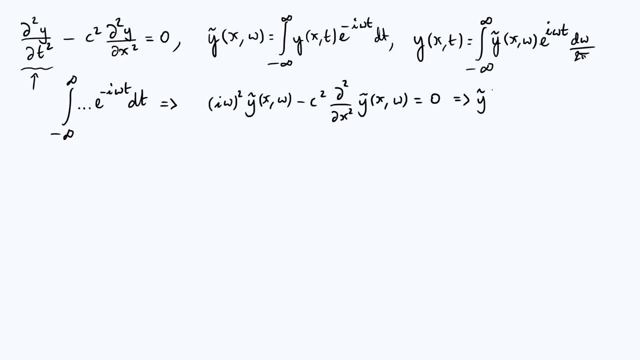 just write the Fourier transform as just y tilde, don't have to explicitly write the dependence in. I'm gonna use a double prime for my second spatial derivative there. so our equation becomes y? tilde double prime plus omega over c. all squared times y tilde is zero. 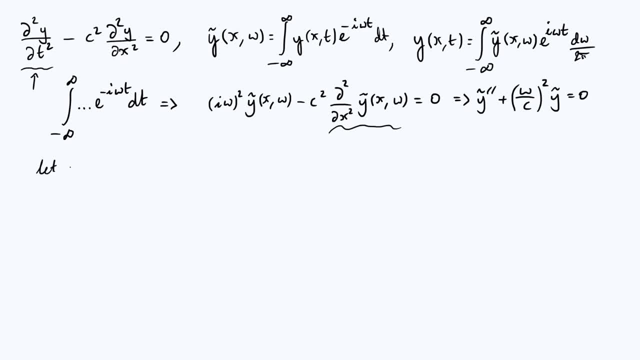 Now it's useful to define another parameter. I'm gonna let k be defined as omega over c and I'm gonna give k a subscript omega, just to emphasize that k is a is really a function of omega. it depends on the value of omega rather than just being a constant. 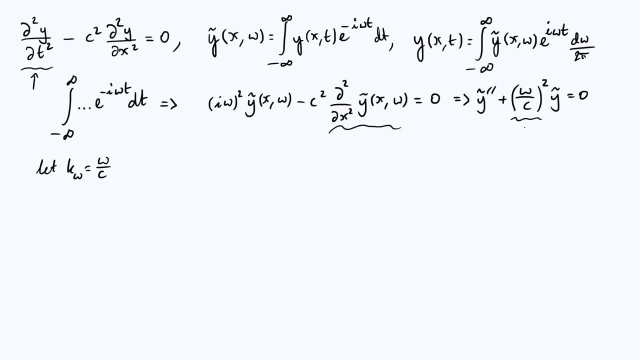 now then this omega over c all squared in our equation. up there is just a k squared, and you may recognize this as just the simple harmonic motion equation, right? so this is an equation that pops up all over the place in physics. i'm not going to derive its solution now, but i'm going. 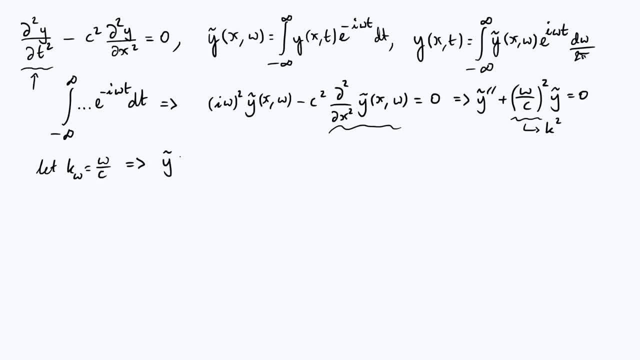 to quote its solution, which is just y tilde, is well, some constant a times a complex exponential e to the i k subscript omega times x, and then some other constant b times e to the minus i k omega times x. now, the only thing we've got to be careful with here is that this double primer is really a. 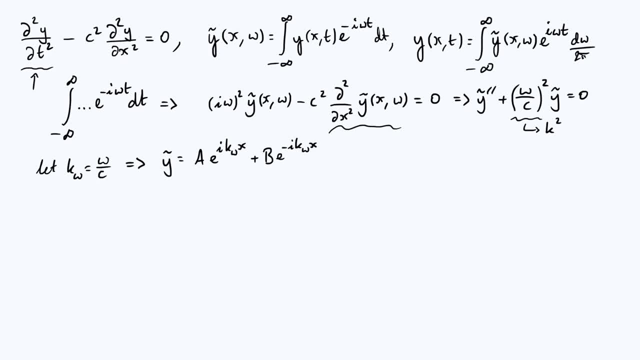 partial derivative, right? so the a and the b here are not actually constants, but they could depend on omega, right? because you know, we just took partial derivatives with respect to x, So those a and b can in this case depend on omega. So we now actually already have a general solution. 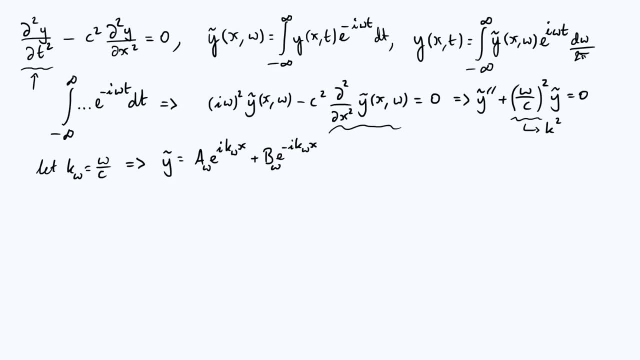 for the Fourier transform of y. okay, a omega and b omega are arbitrary constants. They could be fixed by boundary conditions and initial conditions. but if you're trying to find the general solution, they're just arbitrary constants. So we can go back to y as a function of x and t. 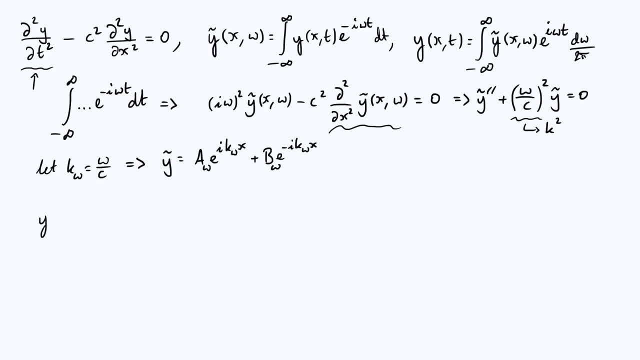 by using the inverse Fourier transform Now. so let's say y of x and t. the inverse Fourier transform was this thing up at the top right? okay, So we need to integrate overall values of omega and equal from minus infinity to infinity. 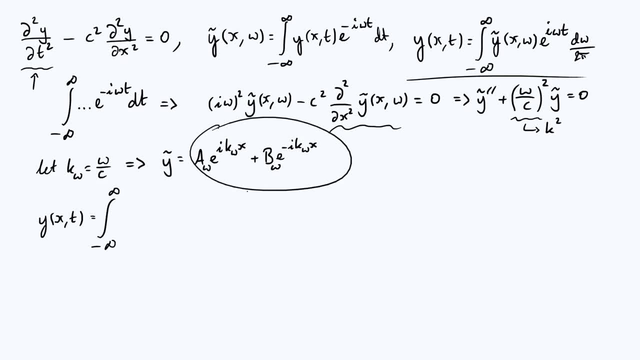 Now, if we take that expression for y, tilde, multiply the whole thing by e to the i, omega, t, as we have to do in the inverse, Fourier, transform. you can combine your complex exponentials together in the following way: right, You're gonna get that first term will be a omega. 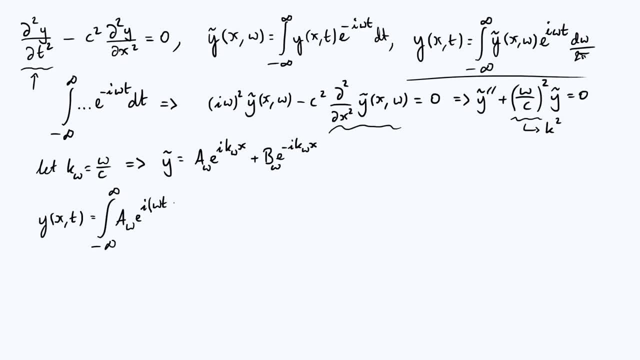 times e to the i omega t plus k subscript omega x. Your second term is gonna be b. subscript omega. times e to the i: Your omega t is still positive, right? That's just part of the definition of the inverse Fourier transform. 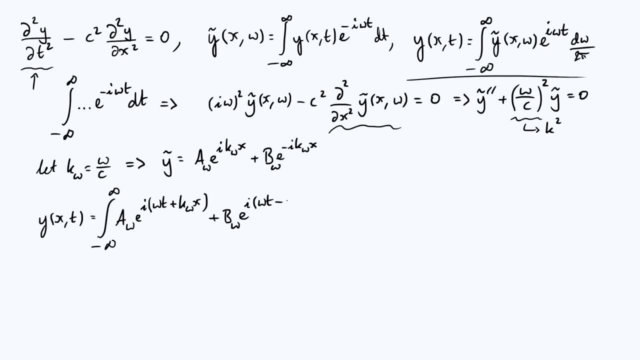 But this time you get a minus sign in the spatial part of your exponent. So it's omega t minus k, omega times x. And then we just integrate with respect to omega and divide by two pi. So now I'm going to split my 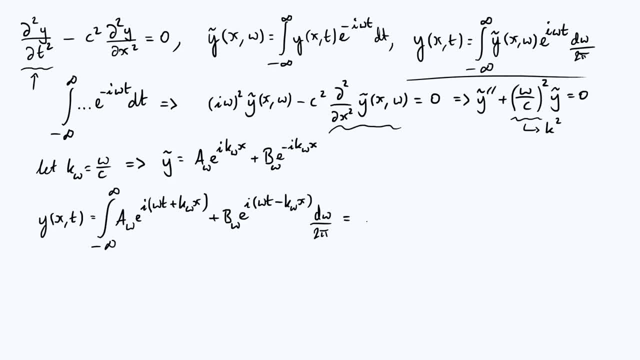 my integral into two integrals. right, For reasons that will become clear in a moment, I'm gonna write as the integral: overall omega, So minus infinity to infinity of a omega. I'm also gonna rewrite my exponent a little bit, So I'm going to write it as i omega. 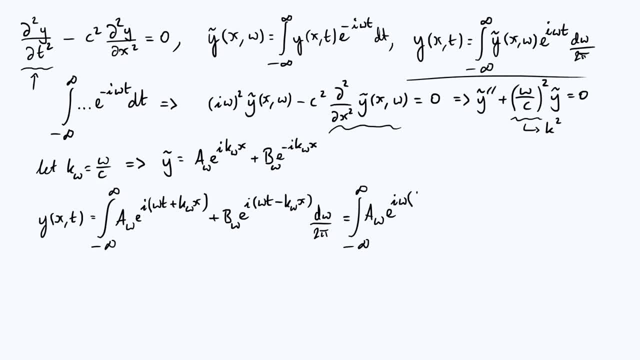 So I'm basically factoring out this omega. Then in my brackets I'm gonna have t plus x over c, which follows from the definition of k omega right, Because k was defined to be omega over c. So if I'm taking this omega out of the brackets there, 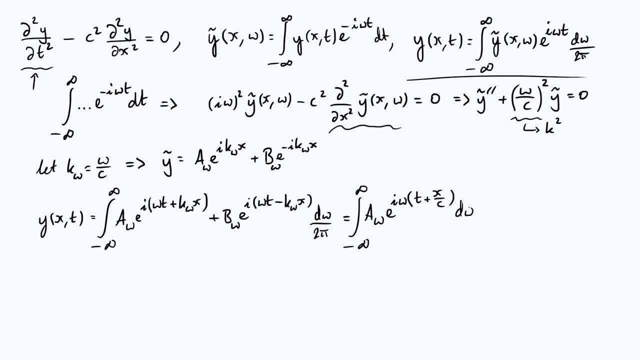 my x is now divided by c, So that is gonna be an integral over omega divided by two pi. And then I'm gonna do a very similar thing for the b part, right? So we're gonna add on the integral from minus infinity to infinity of b omega. 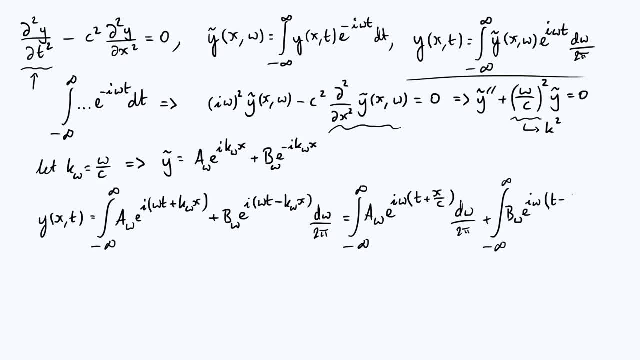 e to the i omega. This time the only difference is gonna be the minus sign. So i omega times t minus x over c, d omega over two pi. So the final step is basically just to notice that each of those integrals is what has exactly the same form. 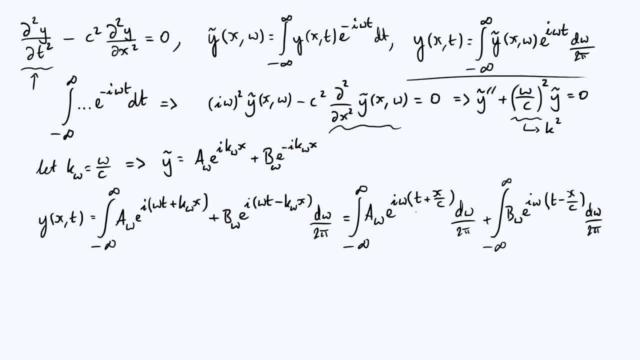 as the integral, you get in an inverse Fourier transform, except instead of i omega t, you have i omega times this combination: t plus x over c in the first one And the second one instead of t, you've got t minus x over c, okay. 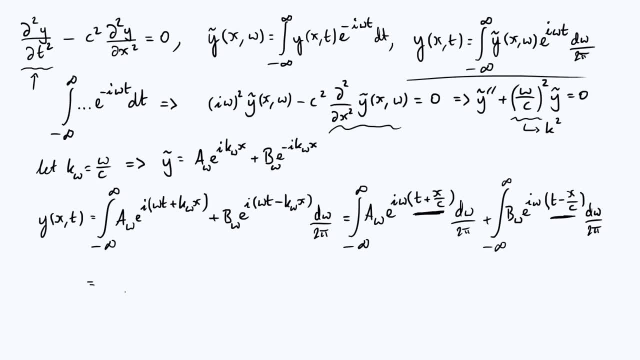 So an alternative way of writing all that, in fact a much simpler way of writing all of that stuff out, would be well, the first integral is just some function right, Some function f, So f of t plus x over c. 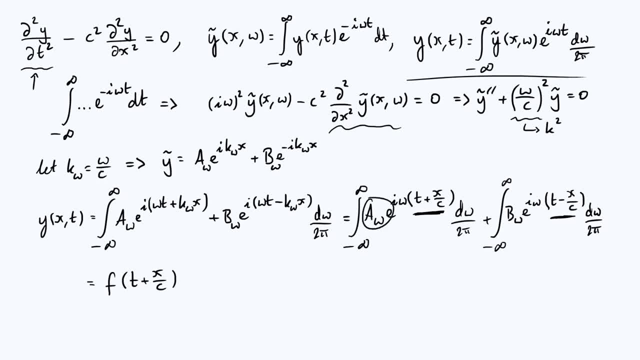 where f is the function whose Fourier transform is a subscript omega right. So it's just any function of t plus x over c That follows directly from the definition of the inverse Fourier transform. Similarly, your second integral is just any function g of t minus x over c. 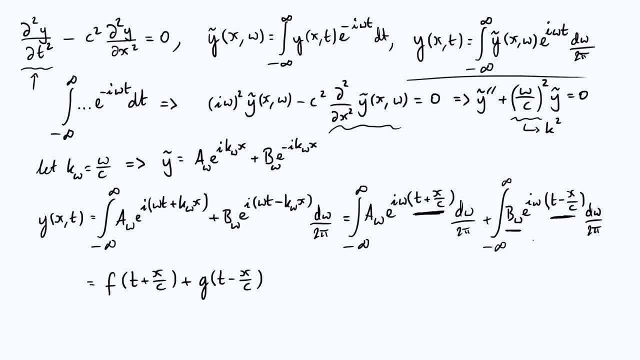 where g is the function whose Fourier transform is this b omega over here. Now, this is already a perfectly valid form of the general wave equation, But let's try to get a little bit more intuition as to what this actually means. Now, to do that, I'm going to factor some constant out of each of the parameters of my f function. 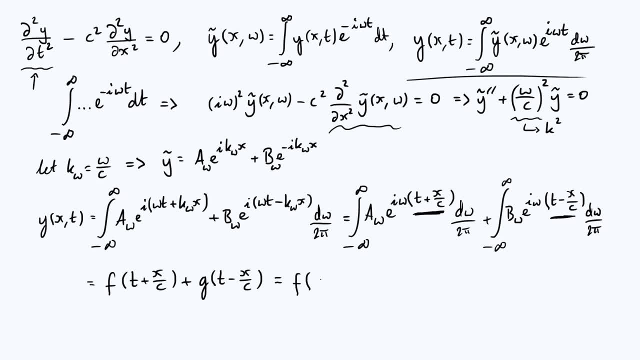 my g function. So for f I'm going to say it's f of c. No, really it's got to be 1 over c times x plus ct, right? The reasons for doing that will become clear in a moment. 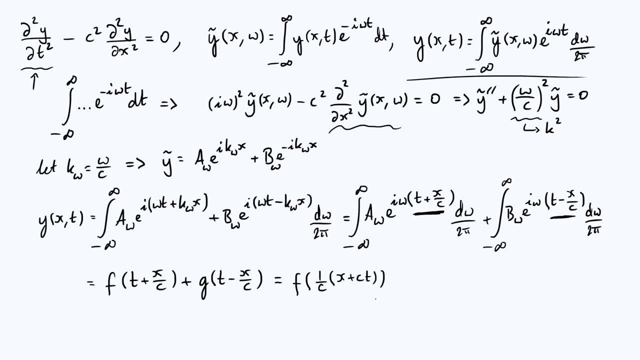 but I'm just factoring out 1 over c. I switched the terms around because, well, the order of addition doesn't matter. So this is completely equivalent to saying f of 1 over c, times x plus ct. Now your second function, g. I'm going to factor out this time a minus 1 over c. 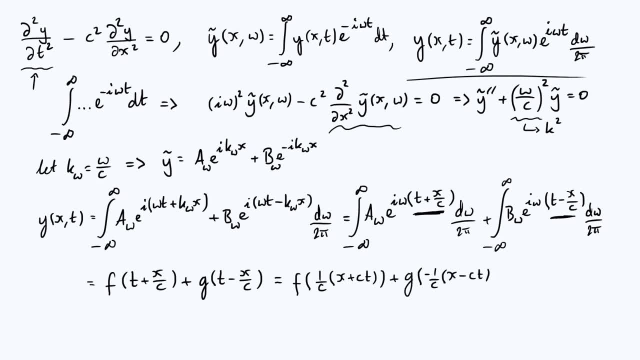 and we're going to get x minus ct this time. Now, this 1 over c and this minus 1 over c are just constants, right, So they're not really important, and you could, in fact, just absorb them. So you could just absorb them. So you could just absorb them. So you could. 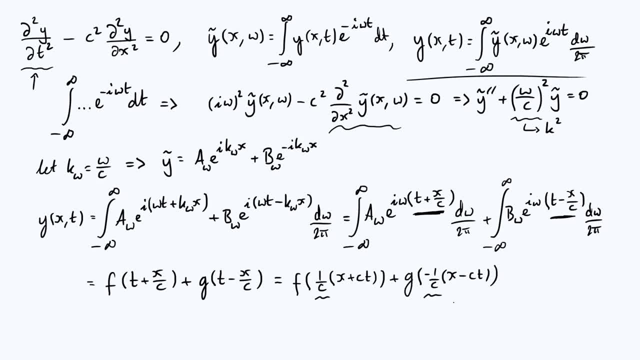 absorb them, So you could just absorb them. So you could just absorb them, So you could just absorb those constants into the definitions of your functions. f and g. right, A function of t plus x over c can be written as some other equivalent function of x plus ct, because they 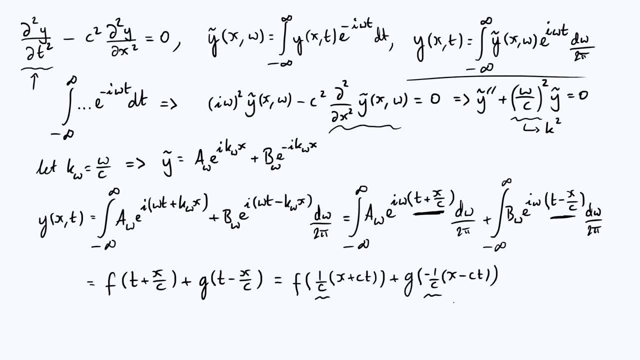 only differ by a constant. Similarly, a function of t minus x over c can be written as some other function of x minus ct, because they just differ by a constant. And so we may as well absorb those constants- 1 over c and minus 1 over c- into the definitions of the functions. but now they're. 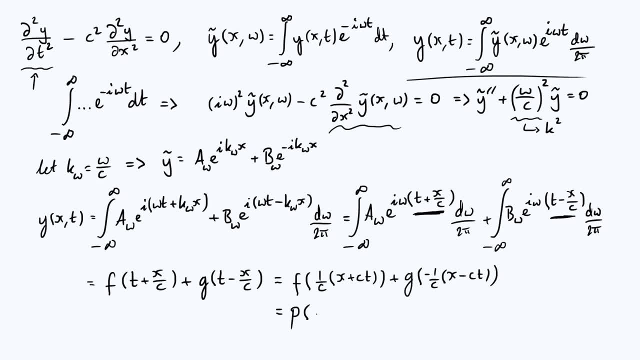 different functions, So I'm going to call them p and q. So another way of writing a general solution is: p of x plus ct, where p is any function plus q of x minus ct, where q is any other function. Now to interpret what this means. 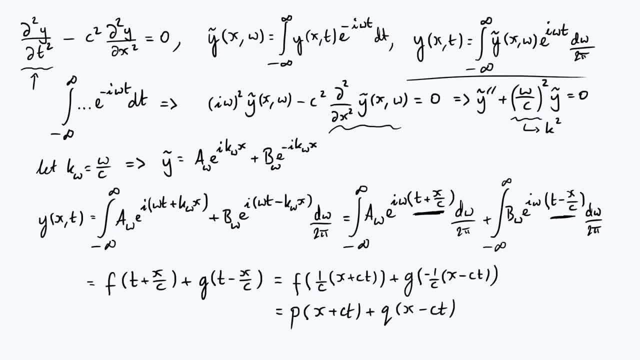 you've got to think about transformations of graphs of functions. Imagine when t is 0,. right, your displacement y is just p of x plus q of x. Now, as t increases um, if you add a positive constant to the argument of your function, that well, graphically, 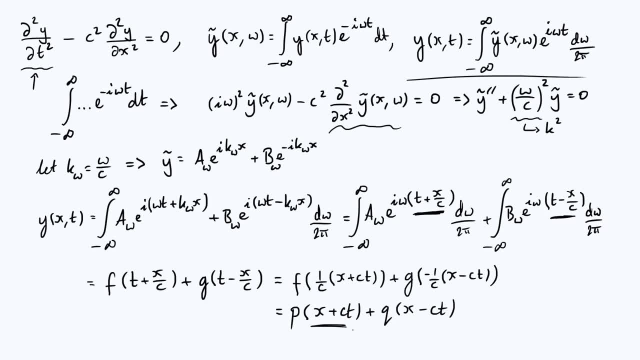 it corresponds to a translation to the left. okay, So as t increases, you're translating your p of x graph further and further to the left. and it's translating at a rate of c right, Because when t increases by 1, you shift your entire function over by an amount equal to c. 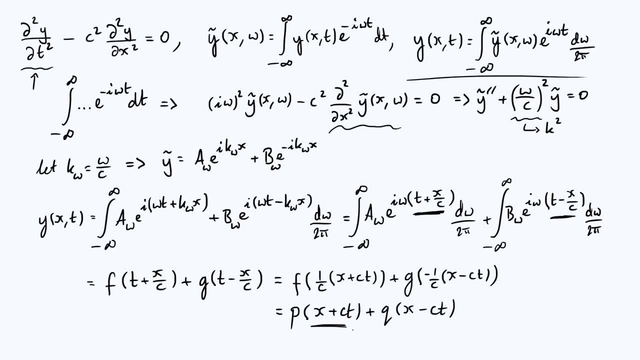 and therefore you're translating your p of x graph further and further to the left. So you're that first part p of x plus ct corresponds physically to a wave right, just some shape moving to the left with a constant speed of c. okay, So the interpretation of c is the wave. 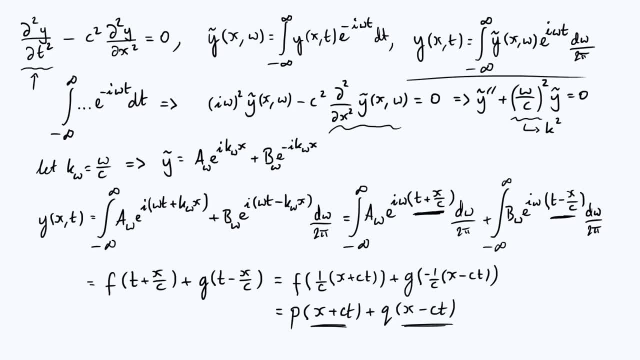 speed. And similarly, if you subtract a positive constant from the argument of your function, that graphically corresponds to shifting it to the right. And again, this time it's shifting to the right at a rate of c right When t increases by 1,. 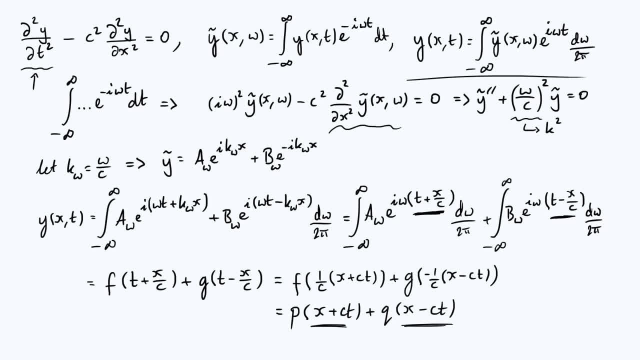 x increases by c. So c is the wave speed again. but the q part of this solution corresponds to any shape, any waveform moving to the right, translating to the right, at a speed of c. So it's basically the solution is just any waveform traveling to the left, superposed with